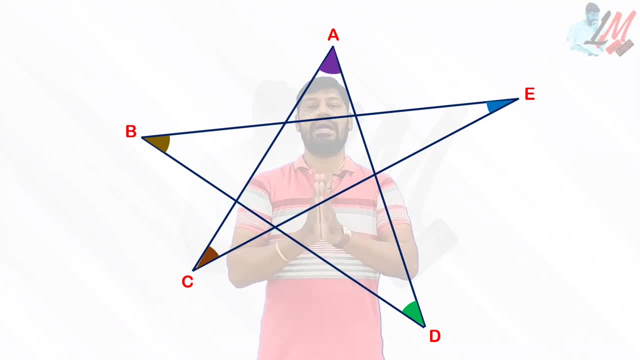 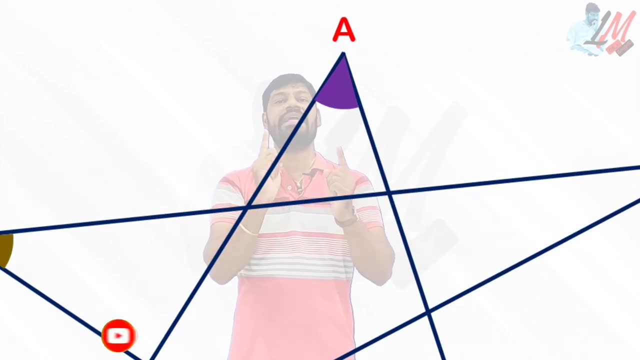 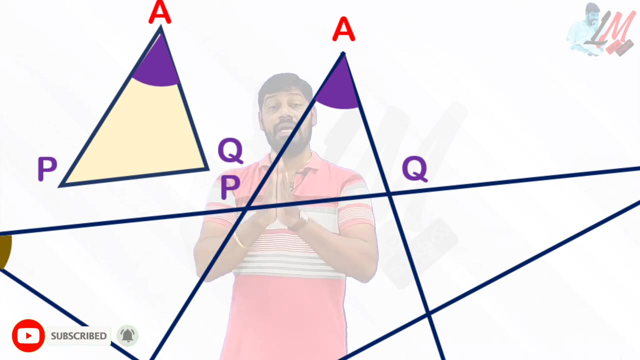 of all the five angles, not individual angles Here what I am doing. so, whatever the vertex is, let me assume this particular triangle and let me take it as this point as P and this point as Q. So clearly you can see a small triangle, A, P, Q here. So if you observe, 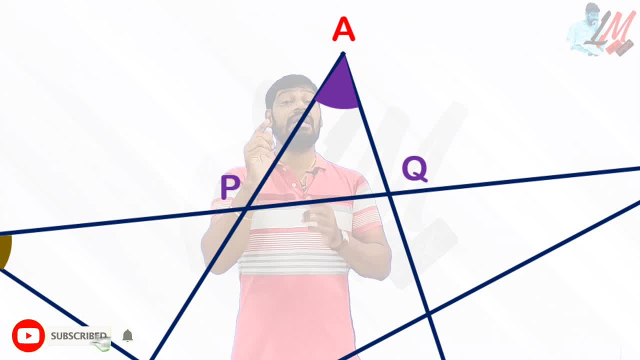 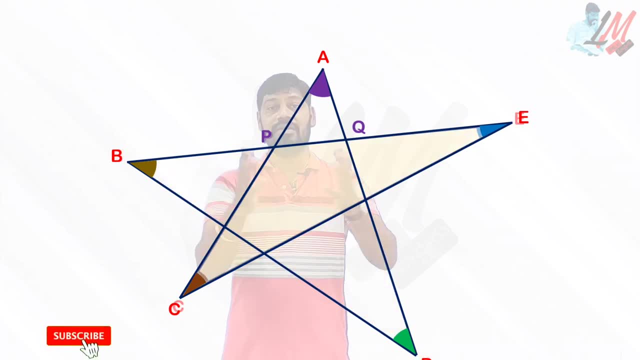 carefully. from point P or vertex P, you can see two different triangles, as P and Q are separate vertices of the two triangles. Have a look at that. triangles here: P, C, E, one to the left, one to the right, one to the right, one to the right, one to the left. 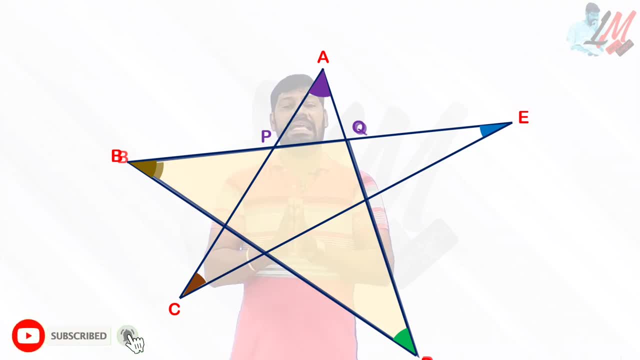 one to the right, one to the left, one to the right, one to the left, one to the right, one to the right, one to the right. Q, B, D: one triangle. So clearly, let me talk about the P C E triangle, only P C E triangle. if you observe carefully, now this CP is extended. 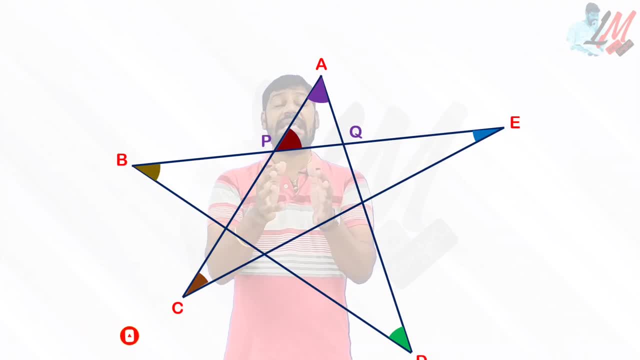 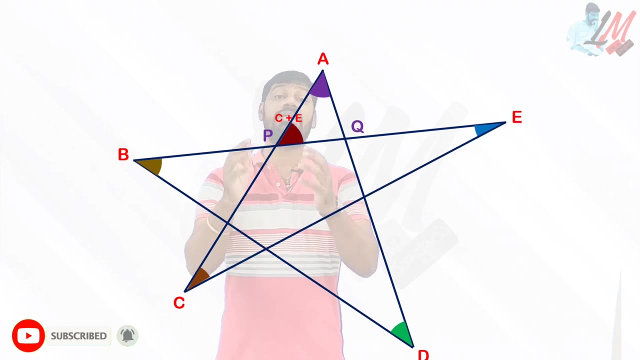 to the vertex A. Clearly, you can see this angle as an exterior angle of particular triangle P, C, E. So then, definitely, this angle is going to be the sum of these two angles. What are the two angles? angle C and angle E? Clearly, you can mention this exterior angle or the 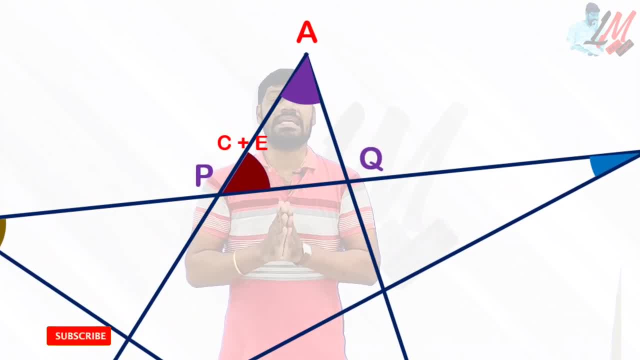 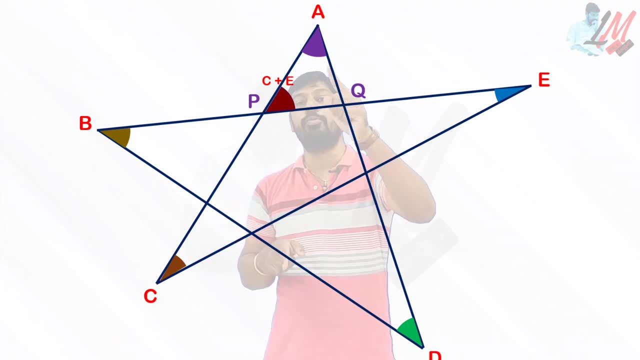 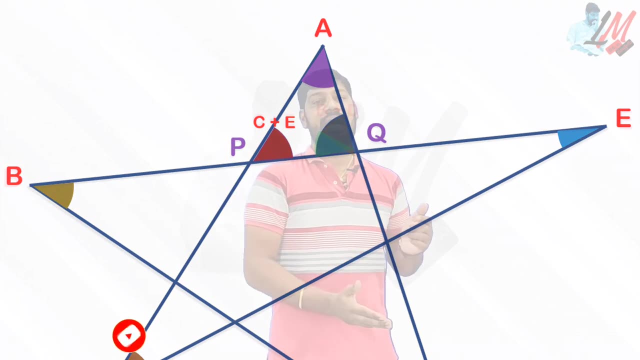 interior angle of this particular triangle as angle c plus angle e. similarly in the triangle q, b, d also. clearly you can see this side is extended up to point a, then definitely this is going to be exterior angle and this is going to be equal with the sum of angle b plus angle. 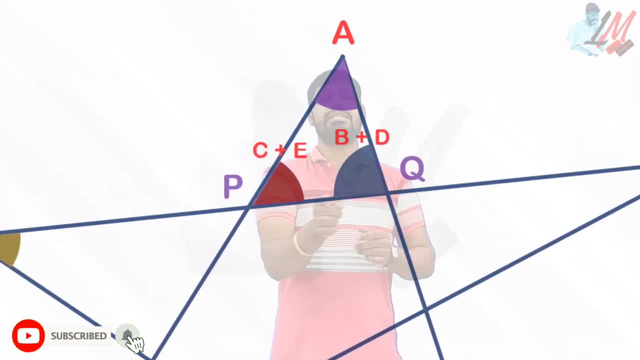 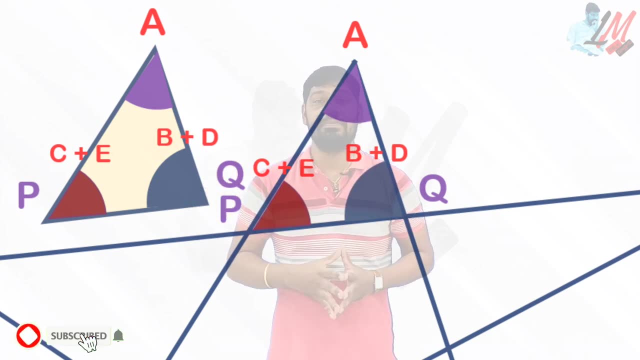 d. clearly you can mention here so simply. you can see a small triangle here in which one angle is angle a, another angle is c plus c and another angle is b plus d. so, as we know, sum of all interior angles equal to 180 degrees. sum of all these angles is going to be 180 degrees on the whole. 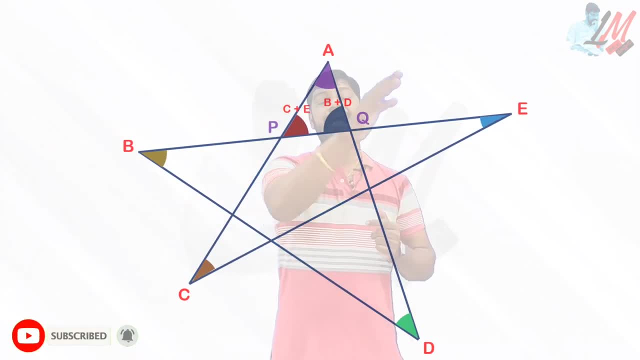 we can conclude in this particular figure, sum of all the five angles is going to be 180 degrees. so simple problem to understand and even the solution. also you can enjoy, like anything, with the help of two basic concepts of geometry, but how you are going to change this one to 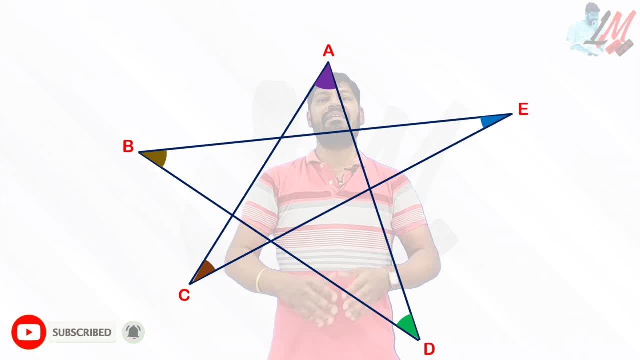 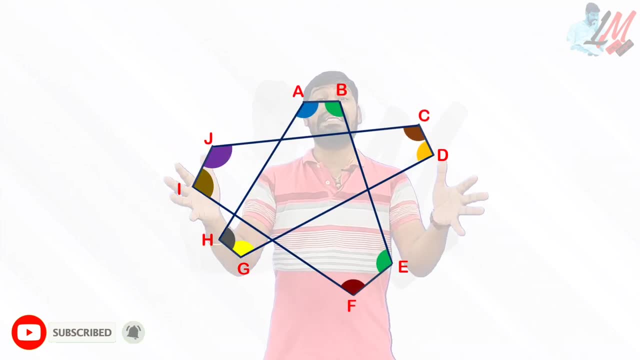 extend the less level of this problem is quite interesting. just have a look. whatever the vertices you can see, just if i cut something like this and i'm going to get a figure with the 10 vertices, what will be the sum of all the 10 angles here? quite interesting. you just give a trial if.